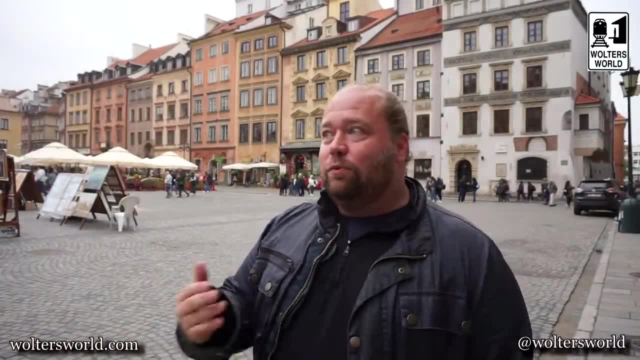 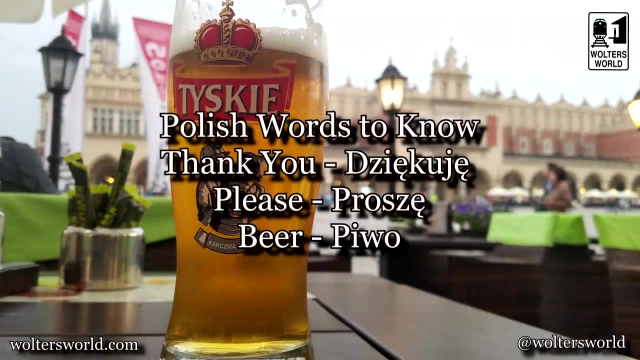 know a few words in Polish. it really opens the door, like people are really happy, even if it's just like dziękuję, which is like thank you, or prosim, which is please, or piwo, which is beer. I remember I was like piwo prosim. they're like. 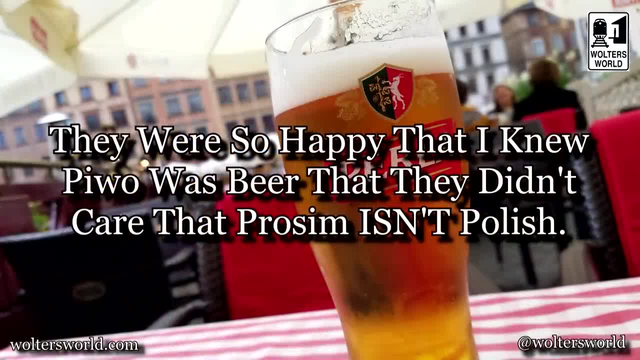 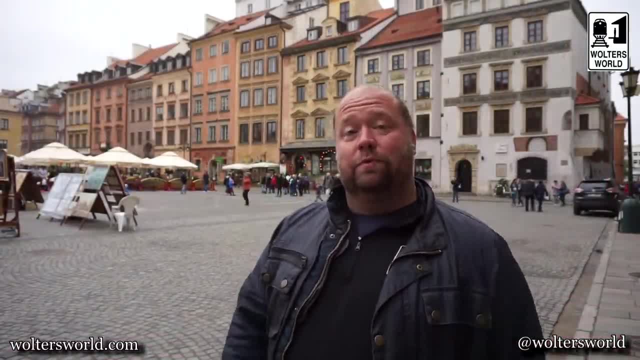 oh, Hey, you know they're so happy with it and it really goes a long way to open up to people because, you'll notice, the people seem kind of dour and quiet and stern sometimes and that's one way to open them up. okay, now our next: don't for. 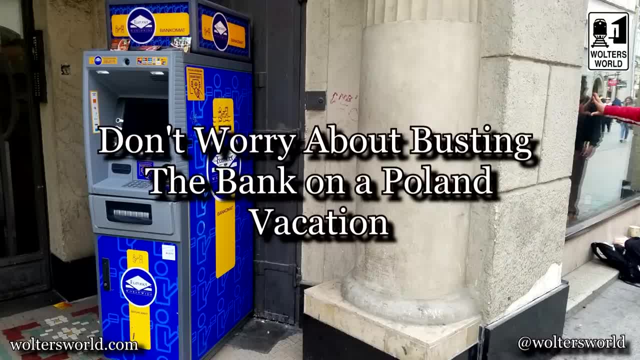 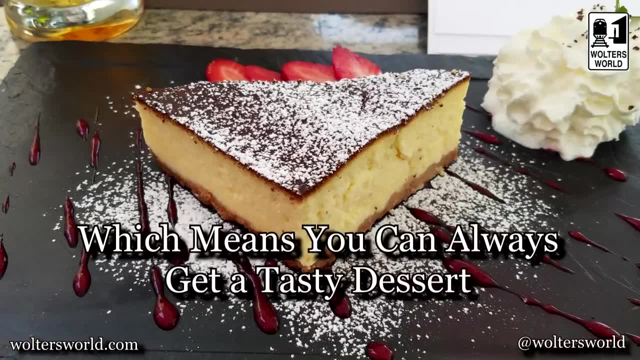 you is. don't worry about busting your the bank when you come here to Poland. Poland is extremely affordable country to visit: hotels, eating, drinking, all kinds of stuff making merry- it is really cheap here. also, going to the museums is really affordable as well, so it's a nice place to check out, that's. 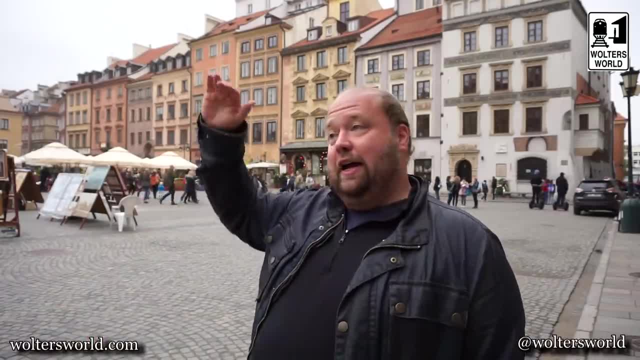 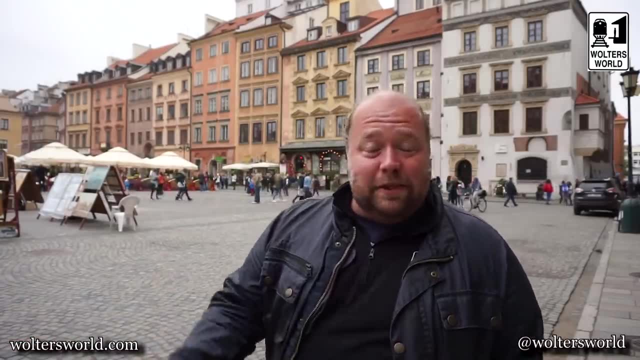 why we you go to Kraków. they get 10 million tours from you know high end tourist to low, low end, low income, not low income. but people aren't spending a lot of money on tourism because it's not a expensive place to be. so that's a kind 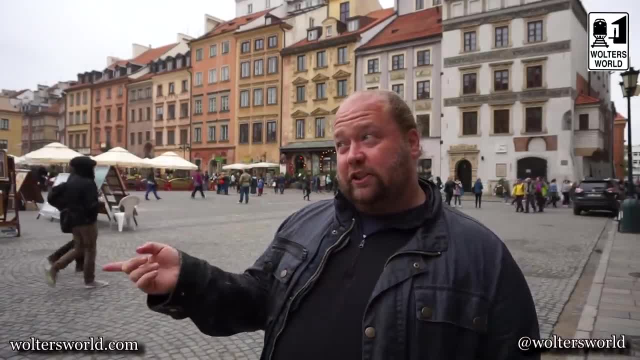 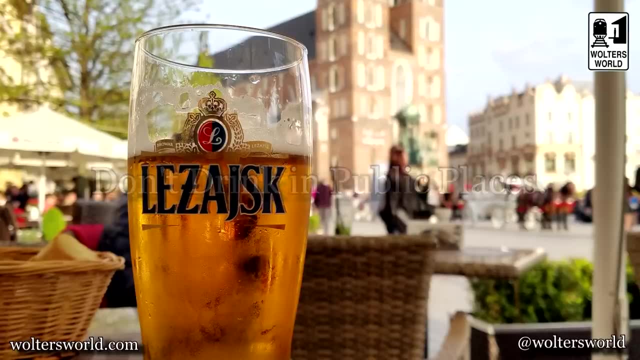 of a cool thing now, if it don't, for you kind of goes along with that cheap eating and drinking. don't drink in public in Poland, look, you can get arrested or fined for drinking in public. now you see this nice square here. yes, you can eat, you drink at the restaurants and the bars, like that. 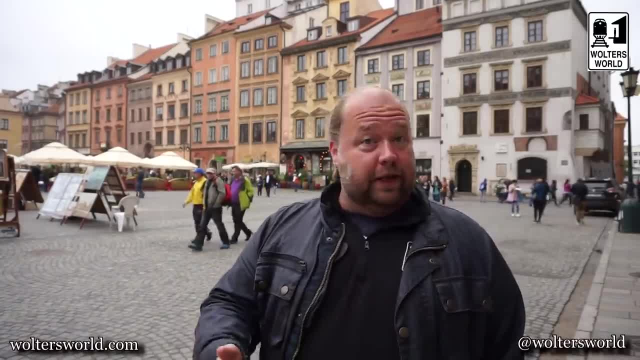 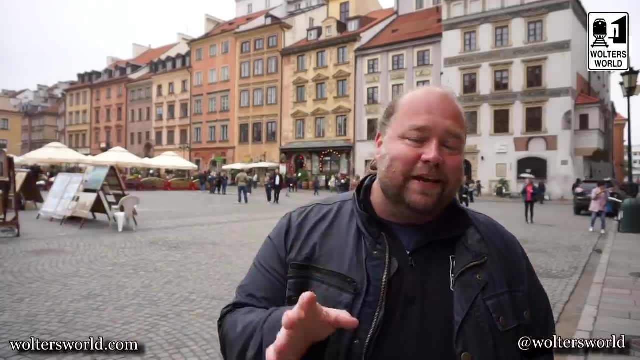 no problem. but if you're gonna like take a some wine, I have a little bit of a or a beer- some of the local beer which are pretty good here and go take that to a park and drink there with your friends. you can get in trouble with the cops, so make sure you do not drink in. 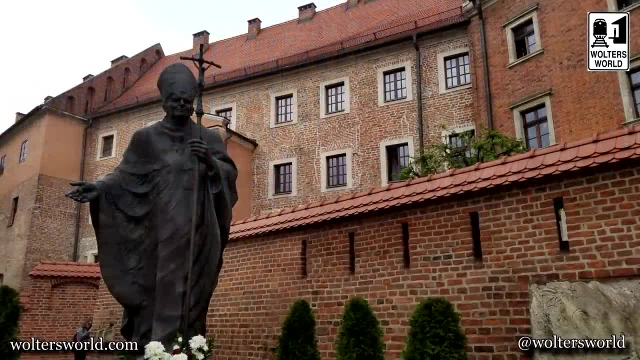 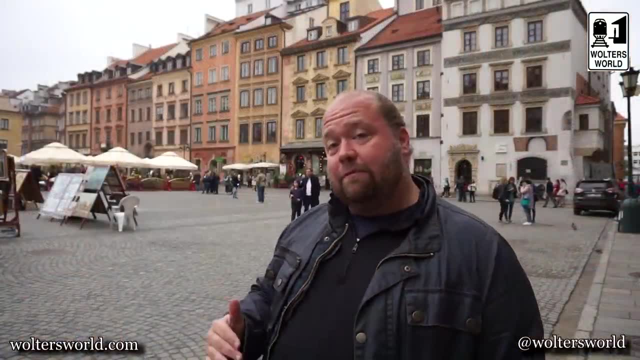 public to go along with that, don't. don't forget, you need to have an id with you all the time. if you don't want to carry your passport with you, what i do is i'll actually have my driver's license from home and a photocopy of my passport, with my passport locked up back at the hotel. so 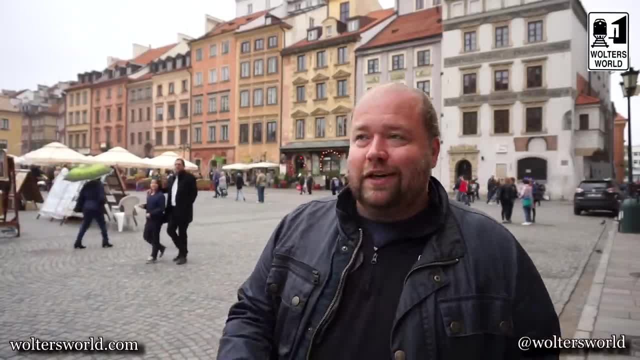 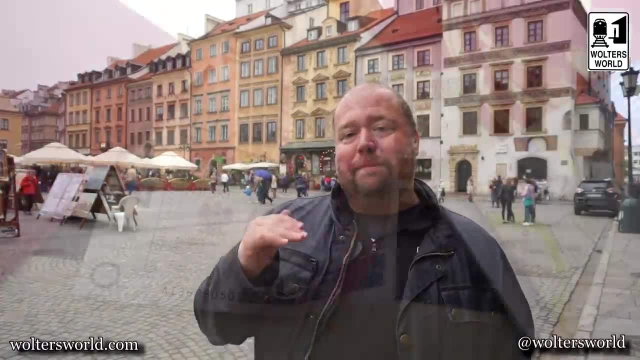 you do have that because the cops could ask you for it if they really wanted to. they usually don't bother the tourists, so it's not that big of a deal, but just in case. so you know. now. our next one for you is: don't try to pay with big bills. now big bills are like 50 swatties or 100 swatties. 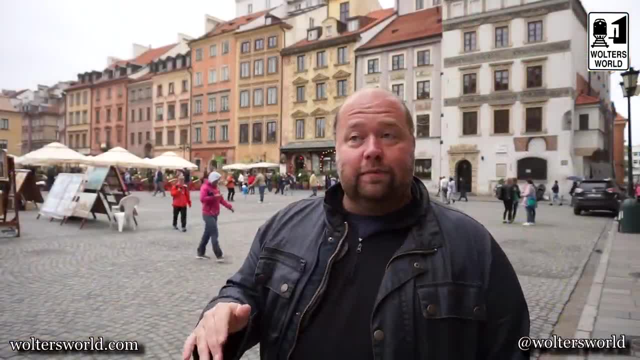 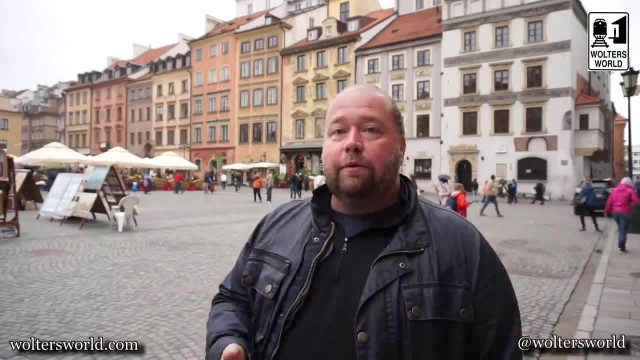 like 100 or 50 if it's like under 20, because people ask you: oh, do you have anything smaller? they're always going to ask for a smaller bill. the thing is, when you go to the atms, it gives you 50s and 100s, but when you go get a beer or something like that it's, you know, seven or eight. i'm like. 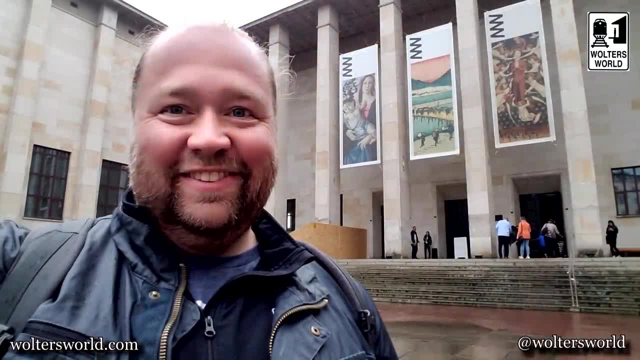 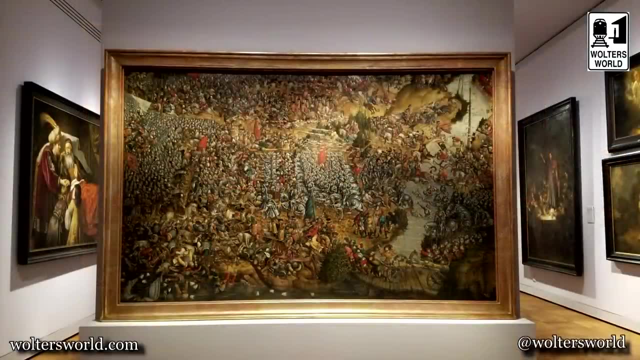 ah, do you have some smaller bills? you have some smaller bills. so when you go to museums, you go to like big stores and stuff like that, use the bigger bills there, the hundreds and stuff like that, to break them into 10s and 20s. so then, 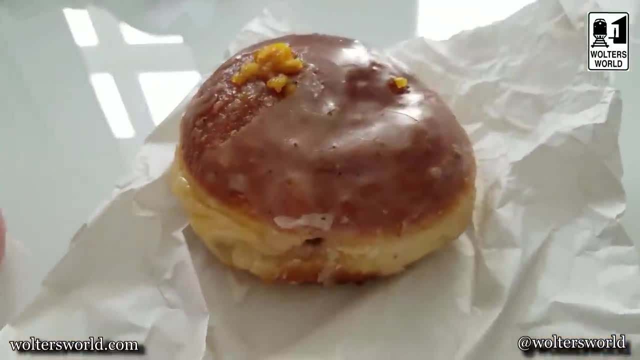 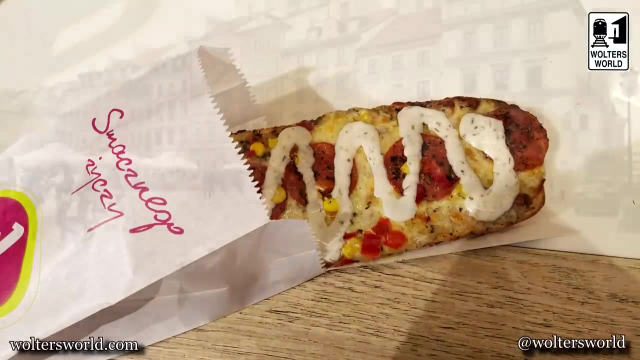 you can go get your little snacks. maybe you want your little- you know- polish donut, or you want to go get a hot dog or something like that when you're here, or just grab a beer. you need that change, okay, so don't use the big bills here right. another don't i have for you is: don't forget to. 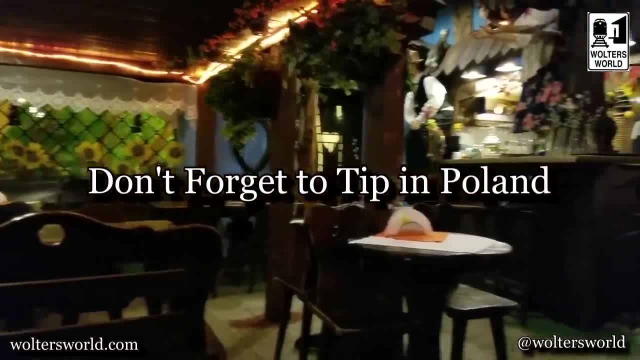 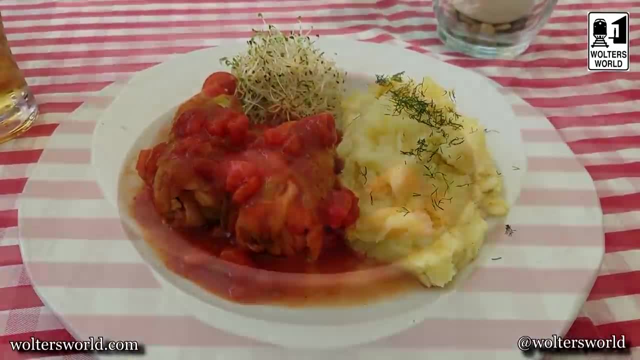 tip when you are here. usually you tip 10 to 15 percent. 10 percent's normal, 15 percent of it's good. but you can look on the menu and some restaurants already put that 10 percent on there. i know the place. i wait here on the square, remember don't. but you're not going to bust the bank. so it wasn't. 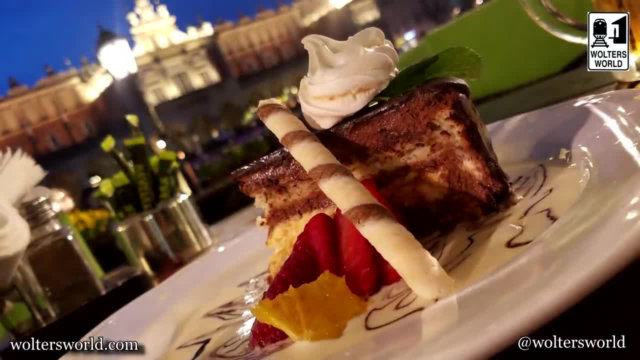 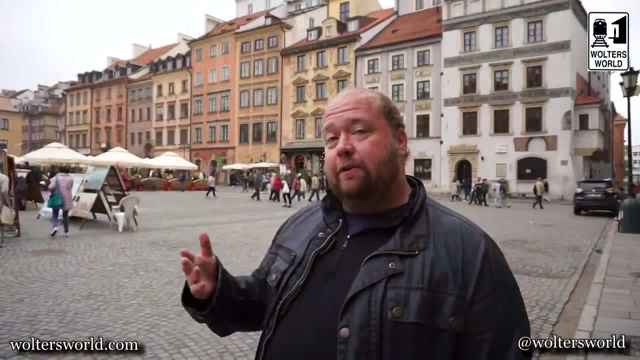 i wasn't. didn't feel ripped off because it was so cheap. uh, the 10 percent was already included. she was very nice and helpful. i gave her a little bit extra on there- no big deal, okay, and going along with that, when you pay your bill, they'll always ask you to play with credit card or cash if you're. 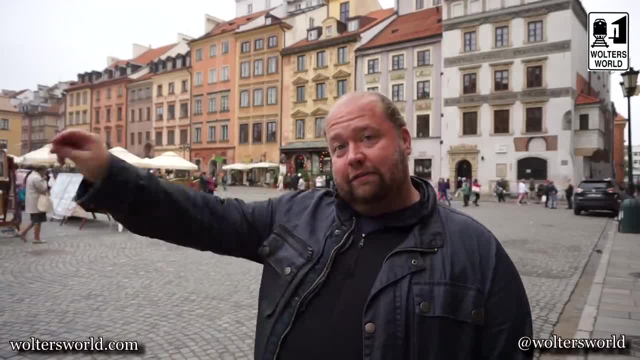 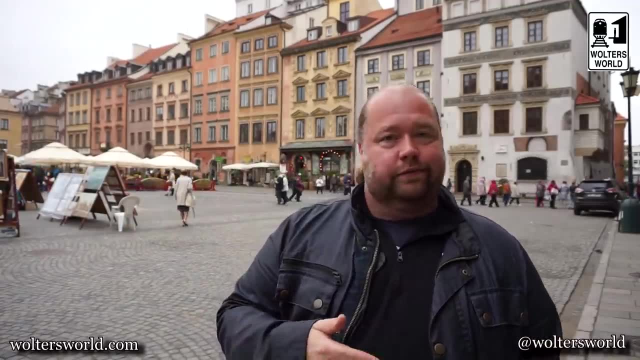 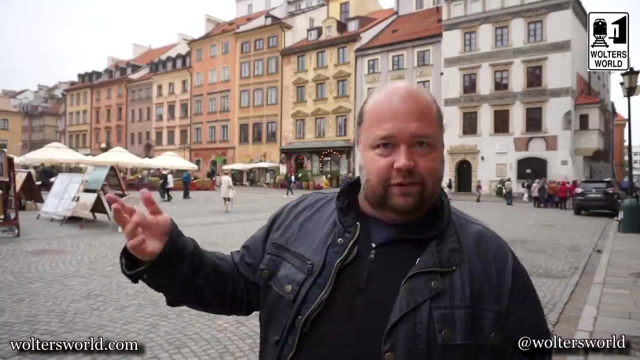 going to pay with cash. if you put the money in the little thing and give it to them, don't say thank you, unless you want them to keep all the money, okay. so let's say you know you got a hundred, hundred and ten 10 bill and you give them 150, you say thank you, or jinkuya, they'll think, oh, a 40, 40, 40 tip for me. 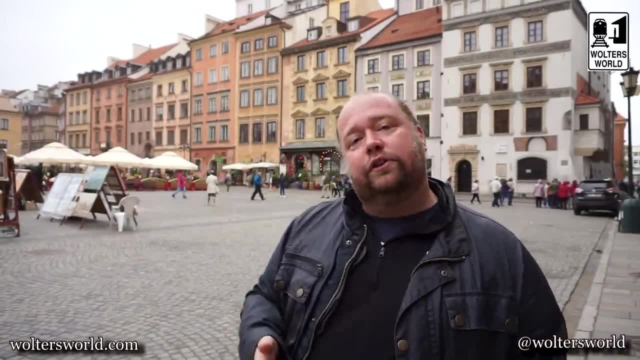 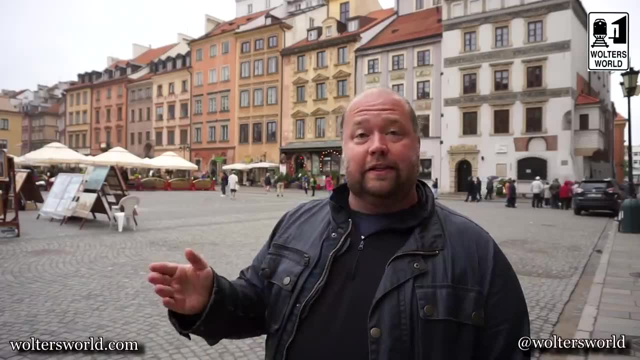 and they'll just walk away with it. you need to tell them: here's this, then they'll bring your change back and then you leave your tip like that. so you have those things there. what i try to do is just have the tip already there. now you might tell them: look, i want to pay 140, and so they'll. 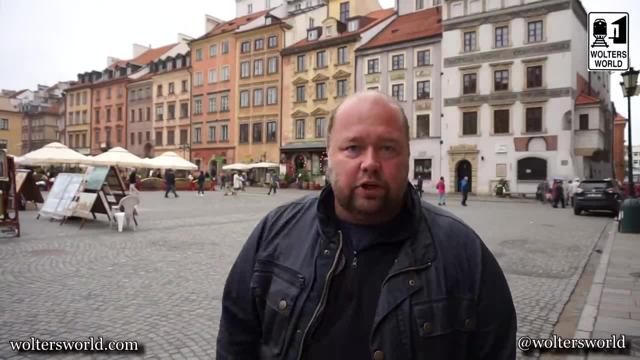 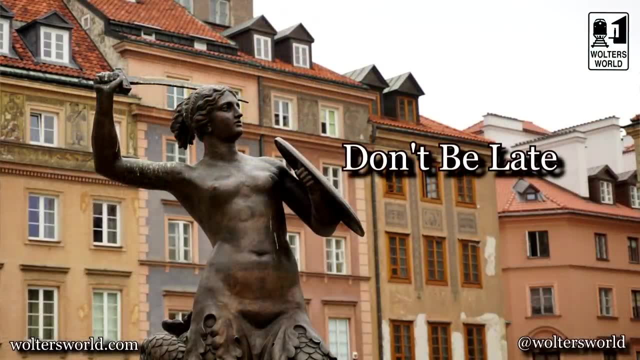 just have the tip from there and give you a 10 back if you have a hundred and a 50, no big deal there. my tenth don't for you is: don't be late. the polls are actually pretty much an on time kind of a type of thing. you know when you're late they're probably late because they're colored, kind of. 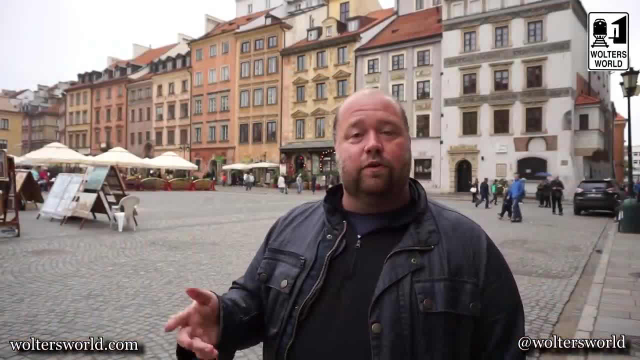 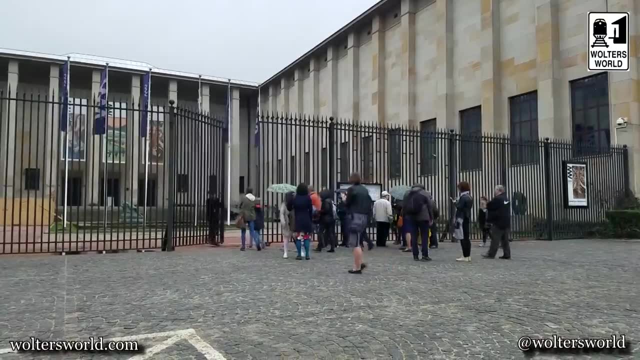 like their german neighbors. if you're gonna be late um to somebody's house you're gonna visit, make sure you call or text them or whatsapp them before so they know you're running behind, because it's kind of rude to be late when you are here. i mean, we were at the muse, i was at the. 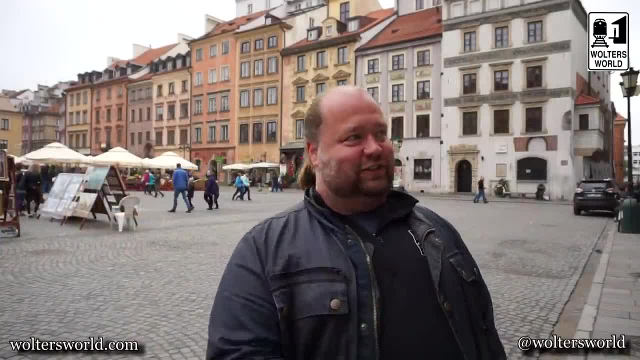 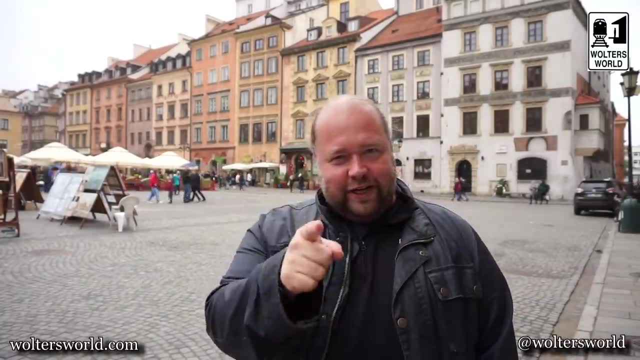 museum this morning and it's supposed to open up a 10. the guy unlocked it like at 1001 and people were like: come on, it says 10 o'clock, let's go, you know. so you do have that there. so make sure you are on time. and my last don't for you is: don't fall for the nature tourism propaganda in poland.